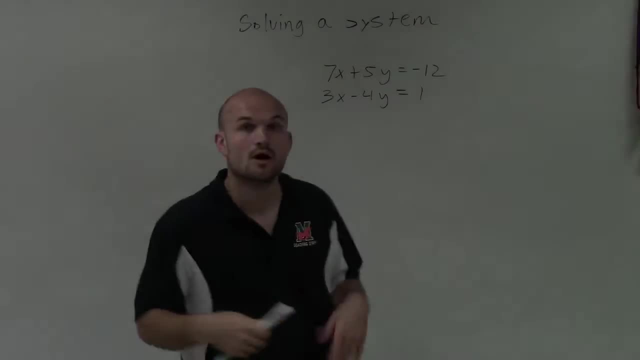 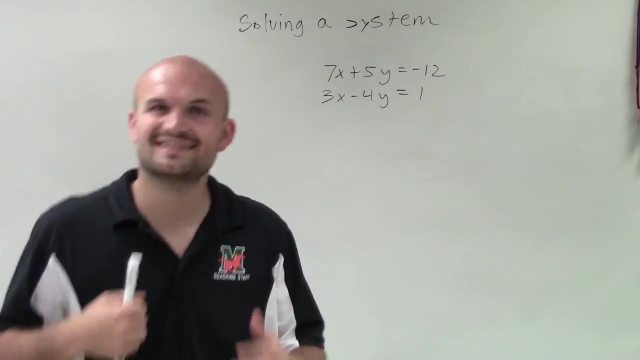 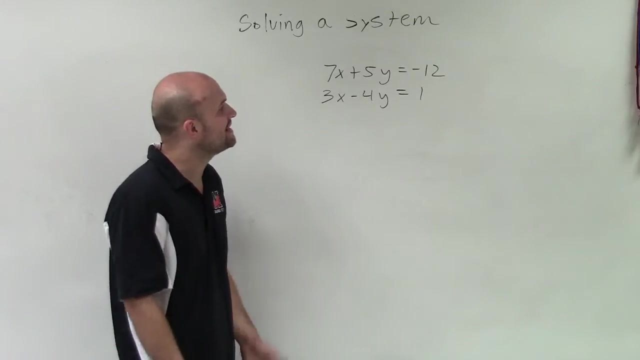 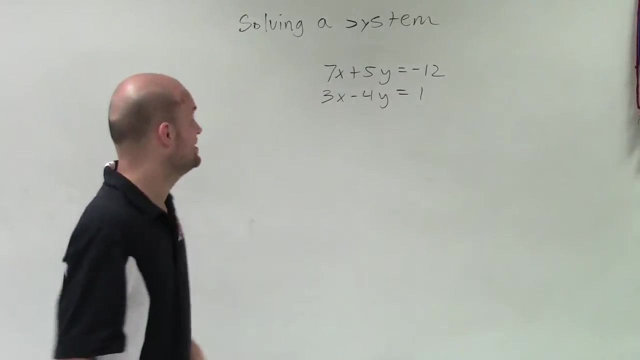 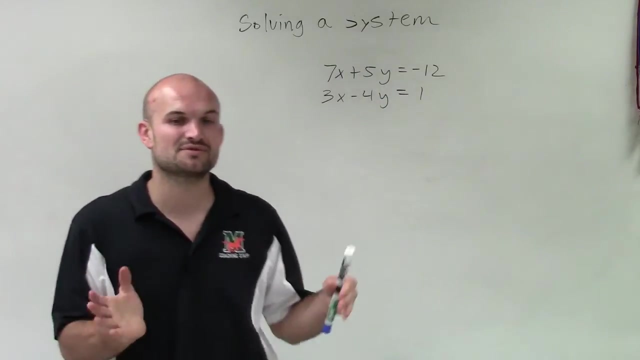 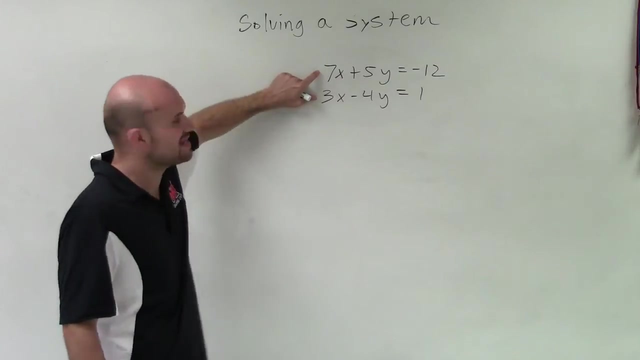 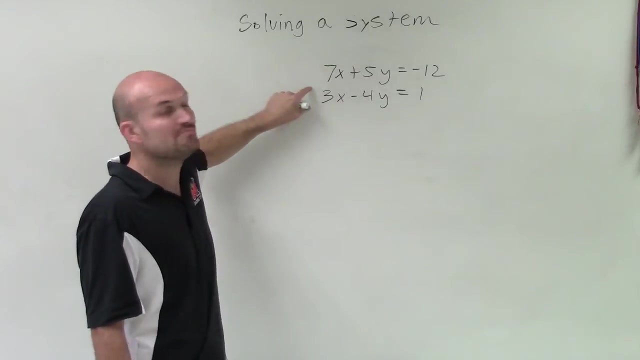 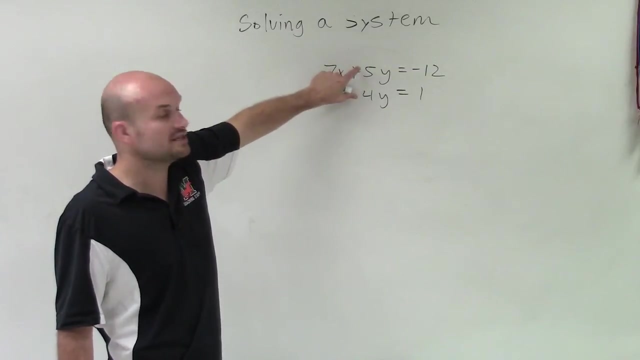 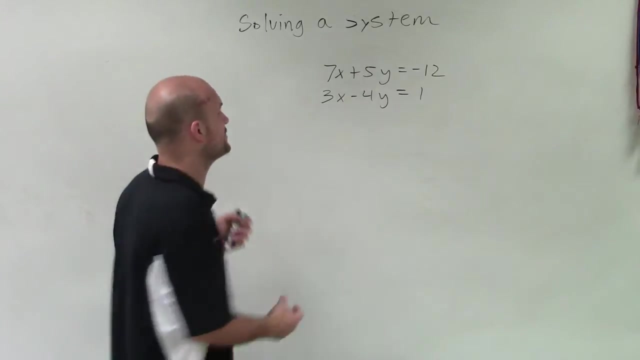 Okay, welcome. So this is one of my favorite types of problems because when we get into, you know, substitution, everybody's kind of like, all right, yeah, I'm getting a substitution. Then elimination, you're like, oh, you know, this isn't too bad. And then, bam, I give you something like this, where now finding the least common multiple of each one of your coefficients is not so outright in front of you, right? So now what we need to do is determine, like, how am I going to find, how am I going to get these coefficients to be the same? Because previously, we've worked with a lot of equations where we only had to multiply a multiplier by one equation. Well, in this case, I noticed that the least common multiple between 7 and 3 is neither 7 or 3, but it's actually 21. So to get to 21, I would have to multiply the top equation by 3 and the bottom equation by 7. Also, for 5 and negative 4, regardless of the negative sign, the least common multiple between 5 and 4 is 20, meaning I'd have to multiply the top equation by 4, and the bottom equation by 5, right? So we have to multiply a multiplier by both equations. Now, it doesn't matter if you want to do 5 and 4 to eliminate the y, or 3 and 7 to eliminate the x. 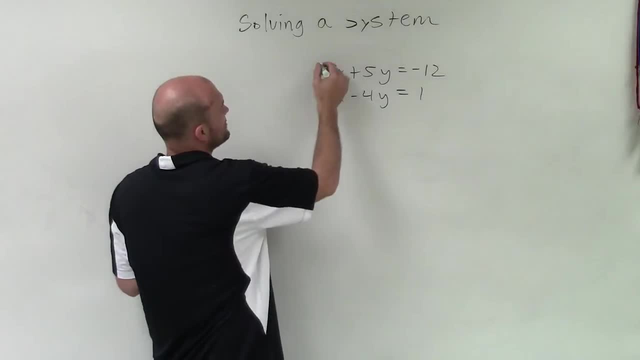 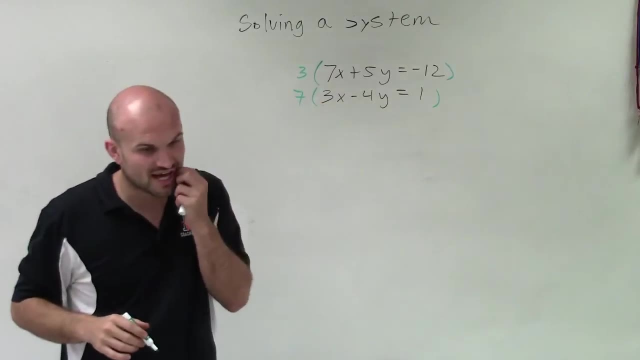 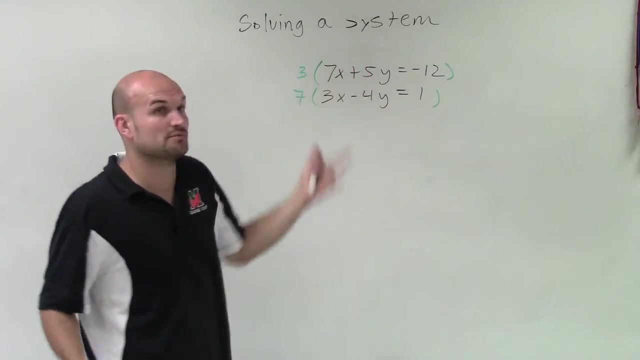 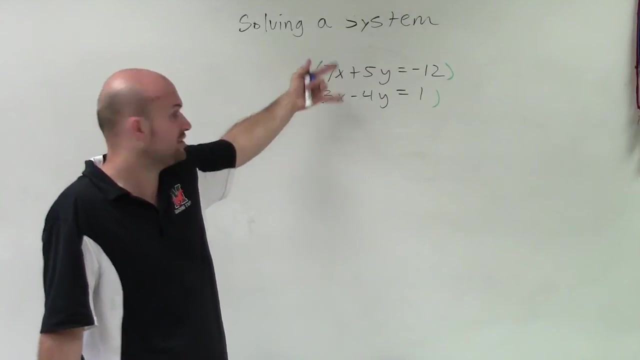 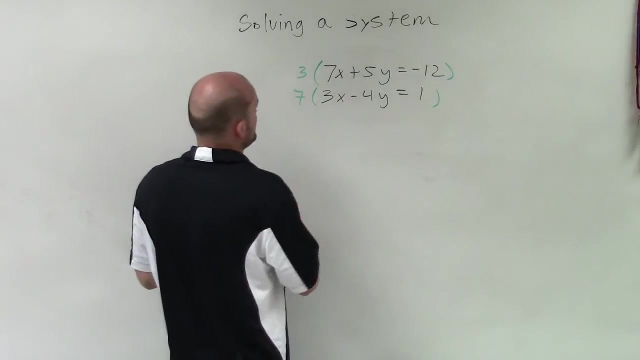 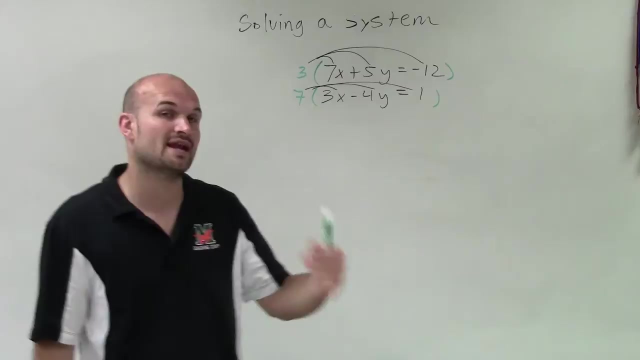 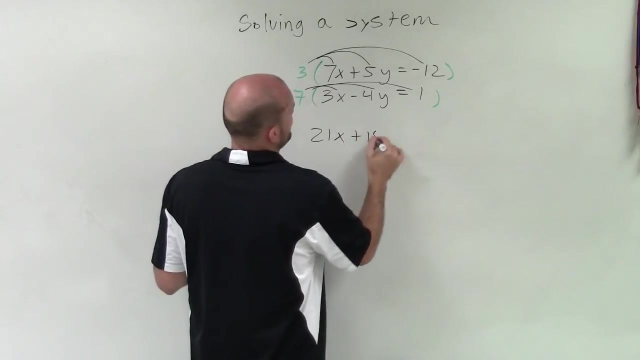 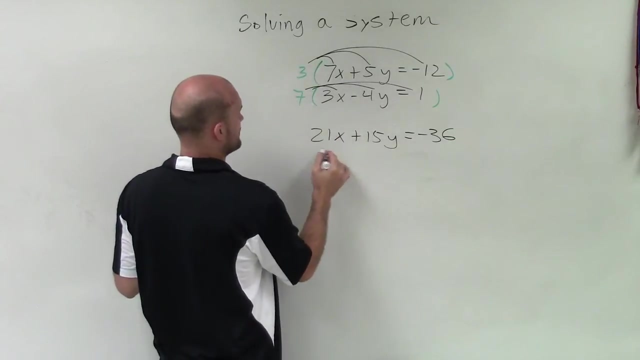 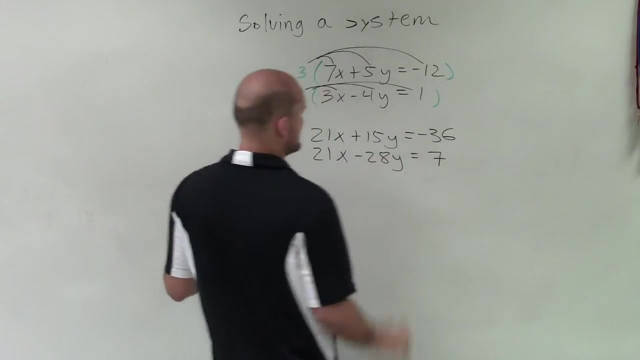 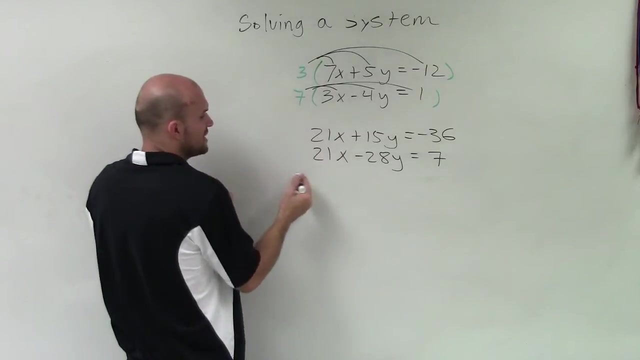 It's really up to your discretion. It's not going to change the answer. But for me, what I'm going to do is I'm going to multiply the top equation by 3 and the bottom equation by 7. And the reason I'm going to do that is because I want to eliminate the x's. Now, notice how the 5 and 4 are positive and negative, right? So if we found the least common multiple, we'd keep them positive and negative, and then we'd add the two equations. Notice how the 7 and 3 are both positive. Now, I can multiply by a negative if I want to, and then add the equations. But if I just multiply by two positives, I'm going to have two positive coefficients, which is okay. You don't have to have a positive and negative, because all that means I'm going to do is now subtract the two equations. So the main important thing, though, is we need to apply distributive property. We need to make sure we multiply everything times our multiplier by every single term, and our equation to produce equivalent equations. And the equivalent equations are going to be 21x plus 15y equals negative 36. And then across here, I'm going to have 21x minus 28y equals positive 7. All right, so those are equivalent equations just multiplied by a multiplier. But what's so important is now we have two coefficients that are exactly the same. 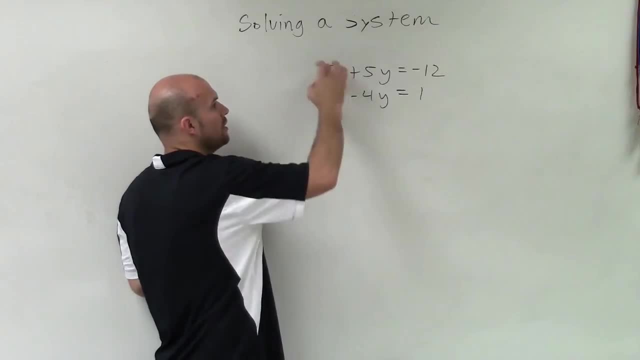 it doesn't matter if you want to do 5 and 4 to eliminate the y, or 3 and 7 to eliminate the x, It's really up to your discretion. It's not going to change the answer, But for me, what I'm going. 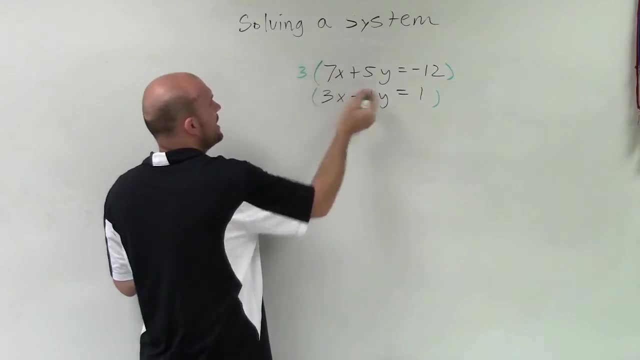 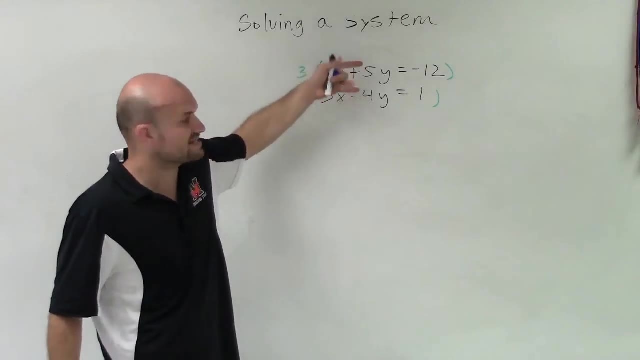 to do is I'm going to multiply the top equation by 3 and the bottom equation by 7.. And the reason I'm going to do that is because I want to eliminate the x's. Now notice how the 5 and 4 are positive. 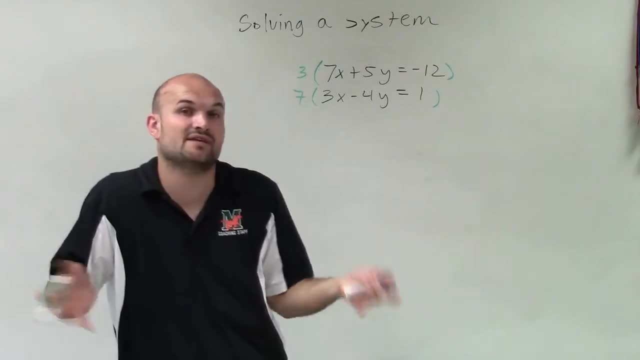 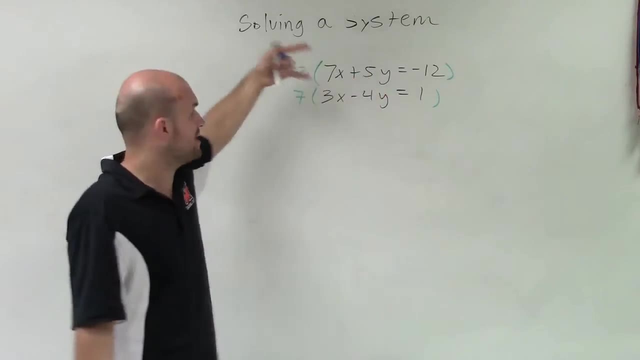 and negative, right. So if we found the least common multiple, we'd keep them positive and negative, and then we'd add the two equations. Notice how the 7 and 3 are both positive. Now I can multiply by a negative if I want to and then add the equations. But if I just multiply, 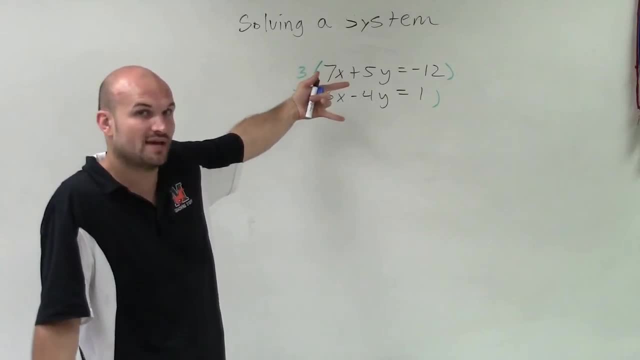 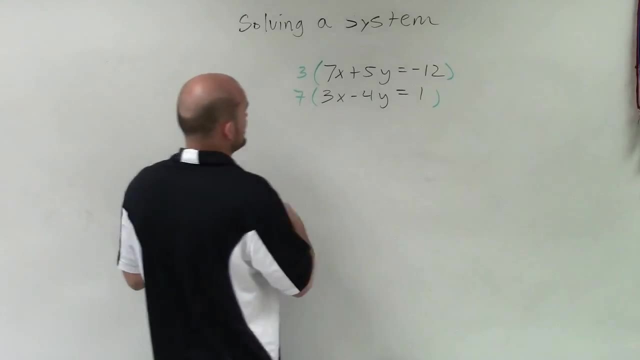 by two positives. I'm going to have two positive coefficients, which is okay. You don't have to have a positive and negative, because all that means I'm going to do is now subtract the two equations. So the main important thing, though, is we need to apply distributive property. We need 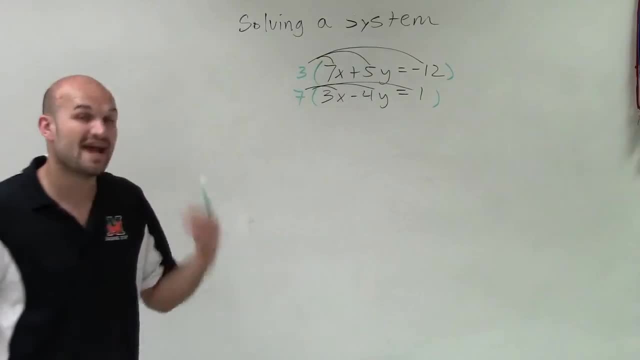 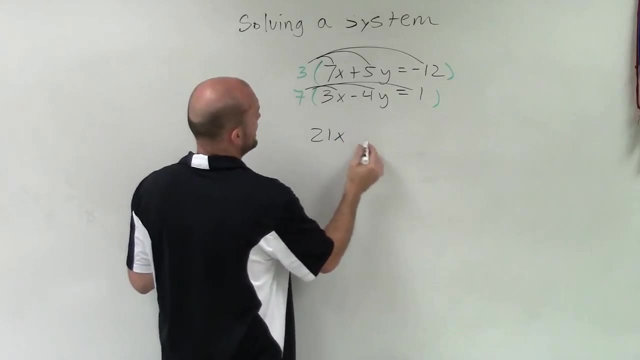 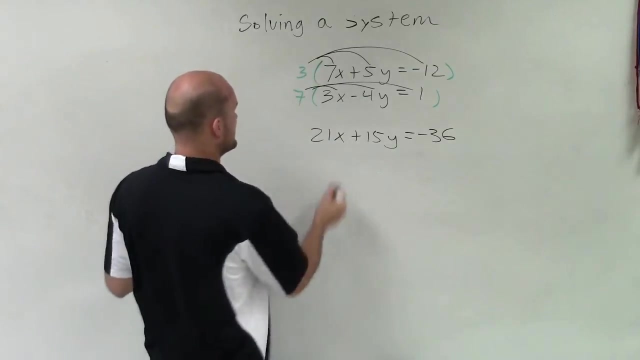 to make sure, we multiply everything, times our multiplier, by every single term and our equation to produce equivalent equations. And the equivalent equations are going to be 21x plus 15y equals negative 36.. And then, across here, I'm going to have 21x minus 28y. 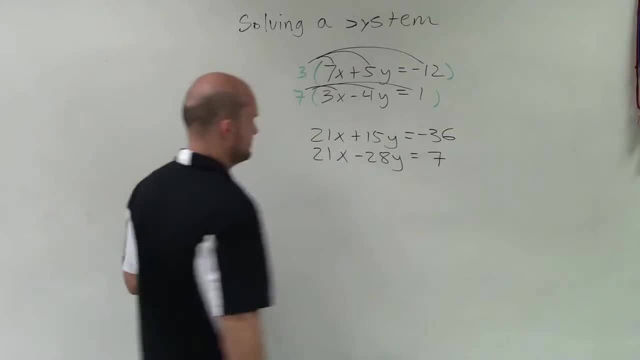 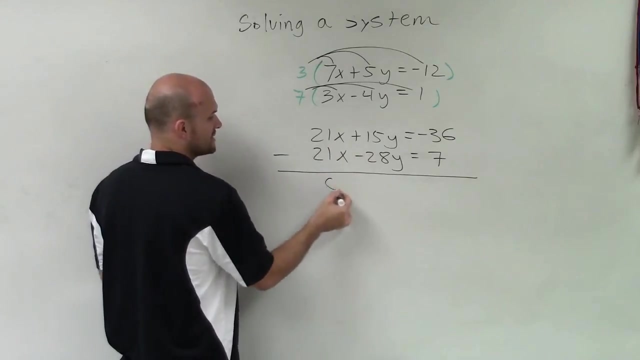 equals positive 7.. All right, so those are equivalent equations, just multiplied by a multiplier. But what's so important is now we have two coefficients that are exactly the same, And since they're both the same sign, I'm going to subtract the two equations, So 21x minus 21x. 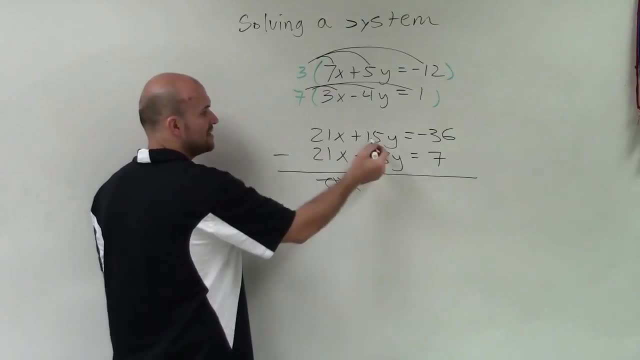 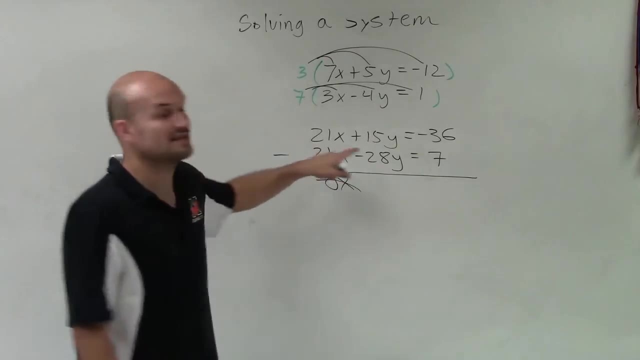 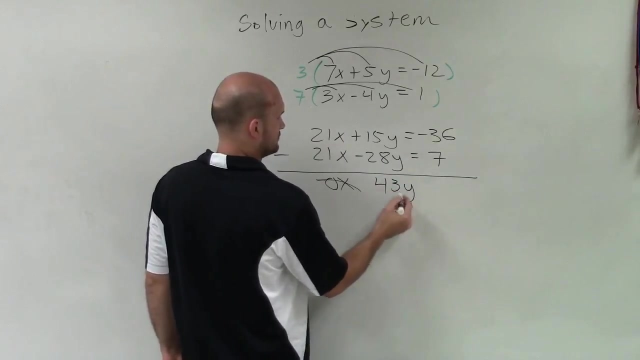 is going to be 0x, which now eliminates my variable x. 15y minus a negative 15y is now going to produce that's going to be a double negative. So that's going to be 43.. 38,, 43. And then negative. 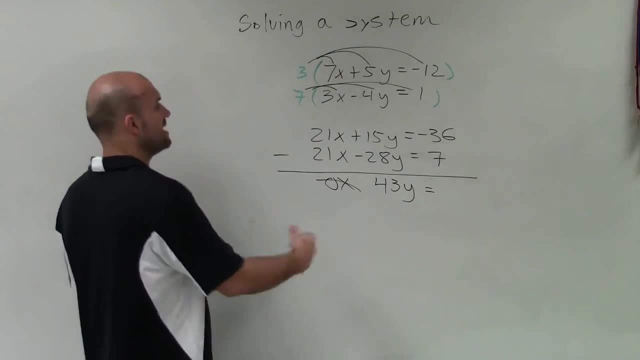 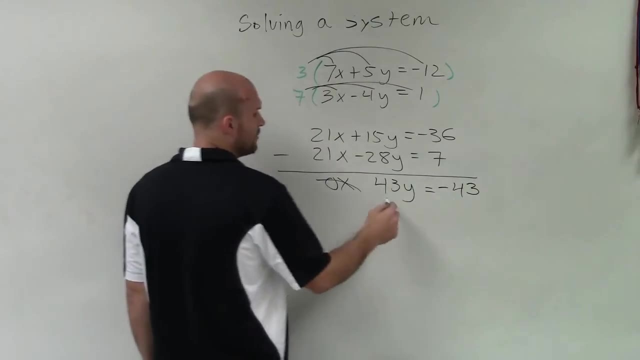 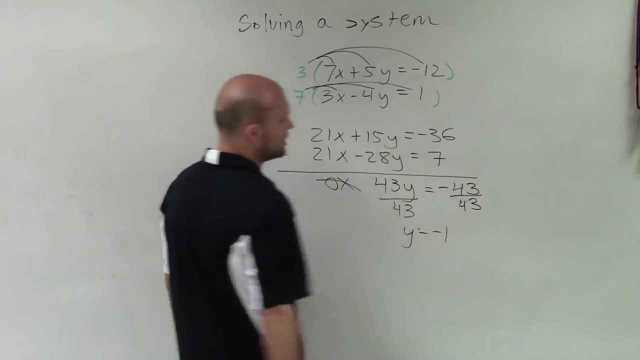 36 minus negative. 36 minus 7 is also going to produce now a negative 43. So now to solve for y: I divide by 43. Don't know what that was- And I get y equals negative 1. So now that I know that,